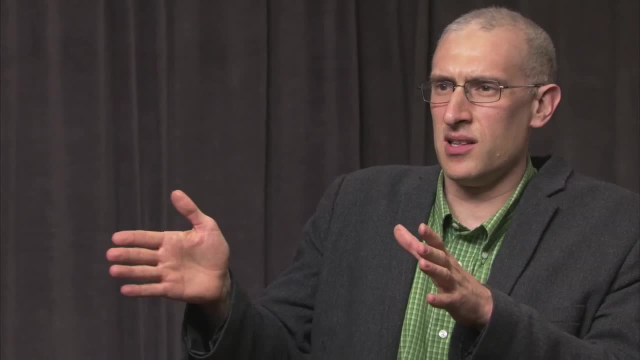 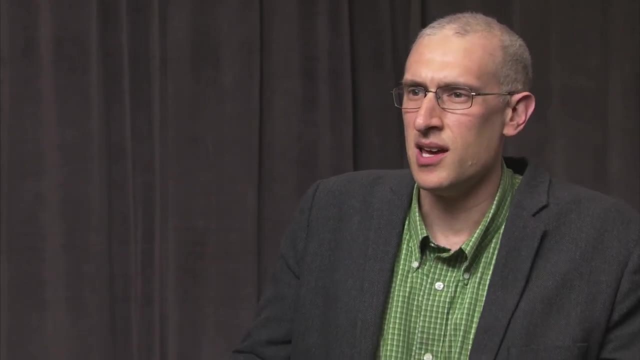 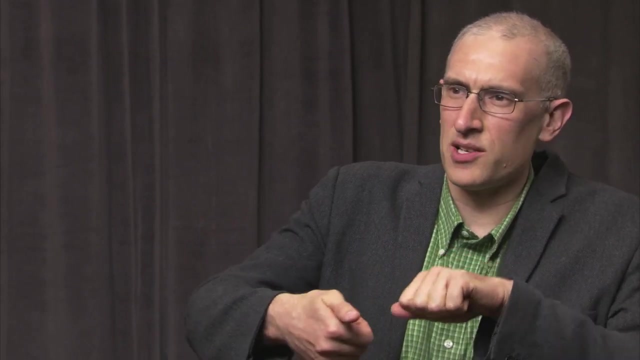 this phenomenal, unprecedented in engineering, attachment system that has these gradients in mineralization, gradients in organization, gradients in composition. But then when you tear your rotator cuff and go to a surgeon, the surgeon goes in and will chop off all of that transitional material and just put it straight down onto bone. It ends up being 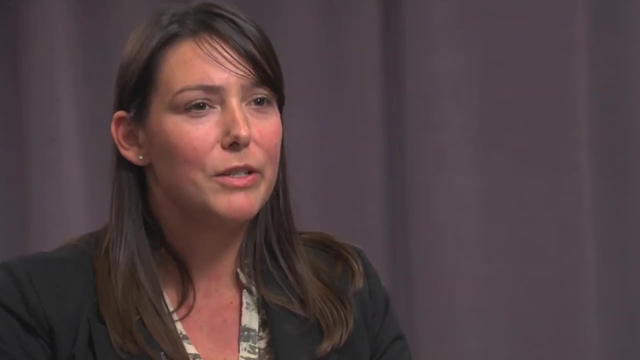 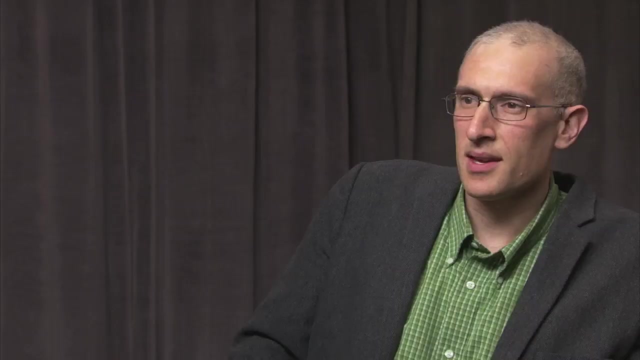 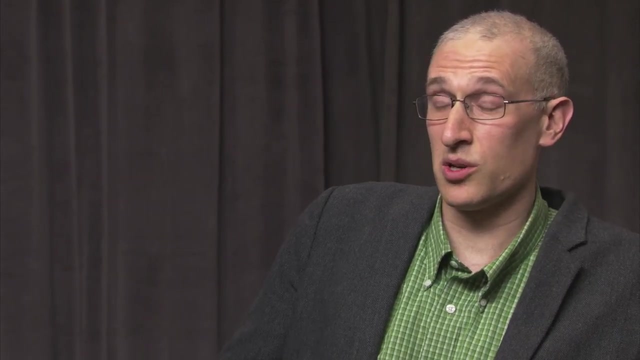 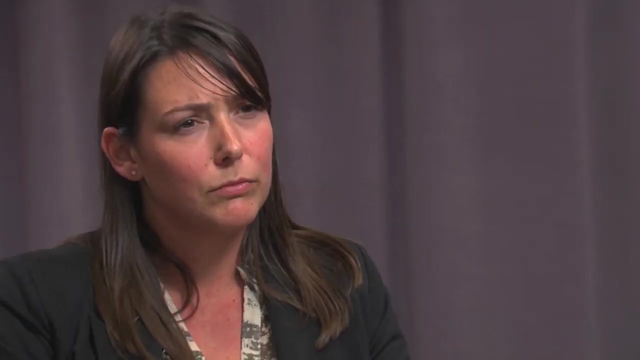 the worst surgery in all of medicine. Yeah, And you see that engineering can step in and fill this gap, this gap left by modern medicine, by surgery Absolutely. And the idea here is that there's some basic physics that the surgical community is neglecting and this basic physics can be used to guide new approaches to surgeries. 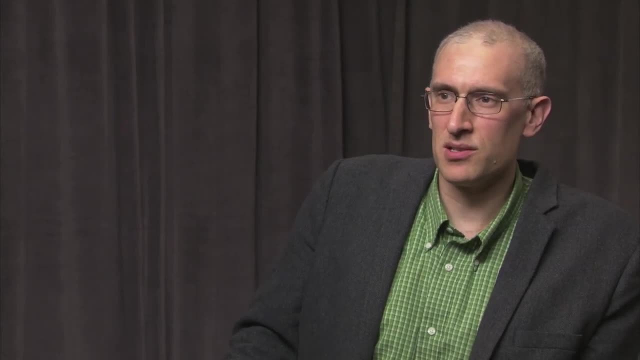 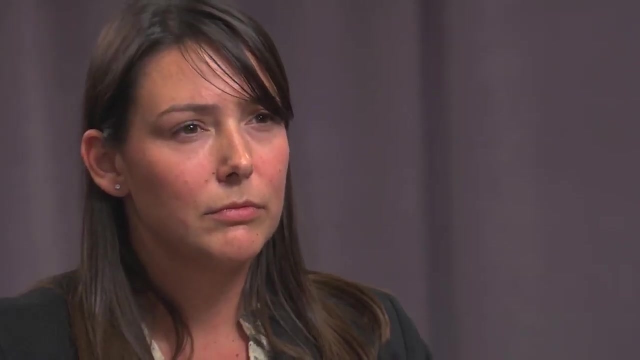 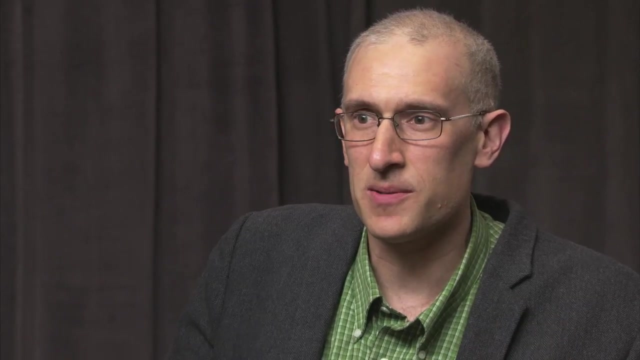 To me, bioengineering is the application of the basic laws of the universe to understand nature and to improve health. Mechanical engineering is the science of relating how structure—structure, following laws of the universe, relates to function, and this is where the next generation of cures lies. 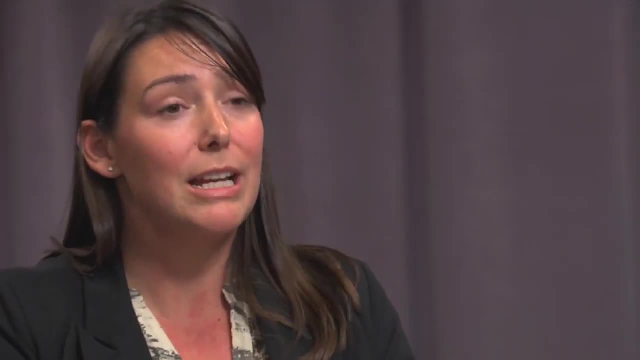 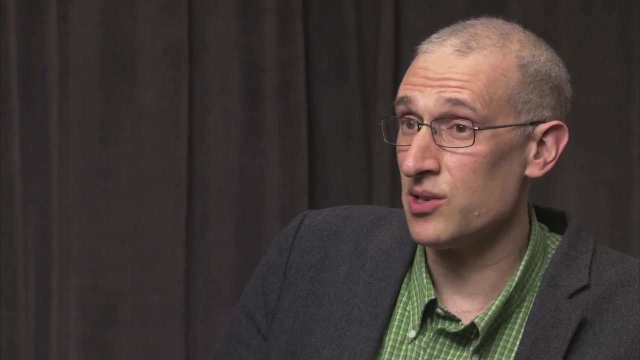 What type of skills do you think the next generation of biomedical engineers needs to have to come up with these next-generation cures, The next generation of cures? what's lacking in the field is the mechanical engineer's background, Mm, Mm. 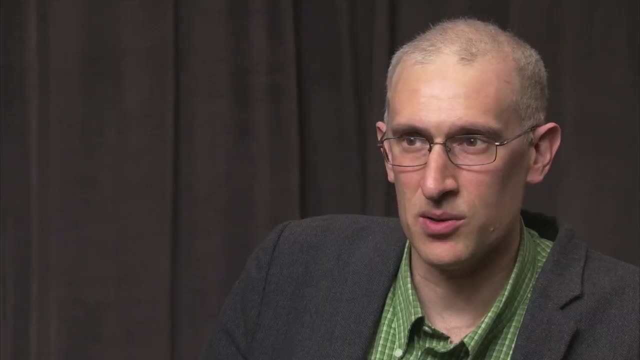 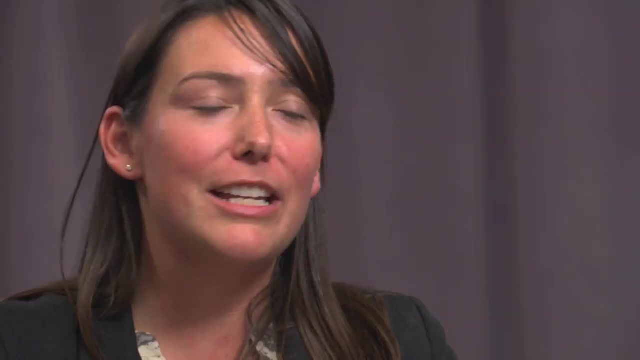 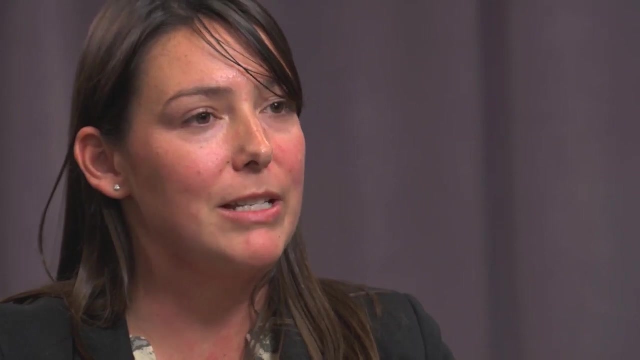 basic laws of the universe, learning how to apply those. learning how to model, learning how to identify what the most important variables are when understanding a system. Can you speak to the value of the interaction and the connection of different levels and different types of engineers coming together through events at ASME to collaborate to? 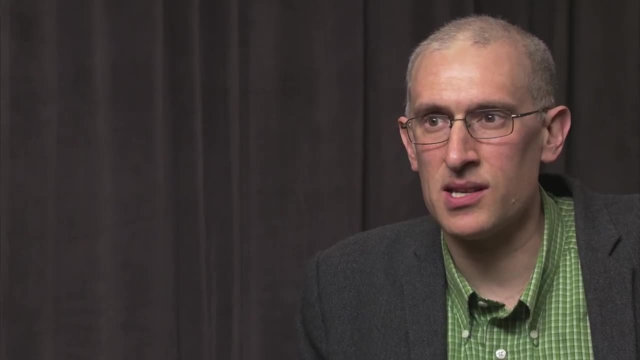 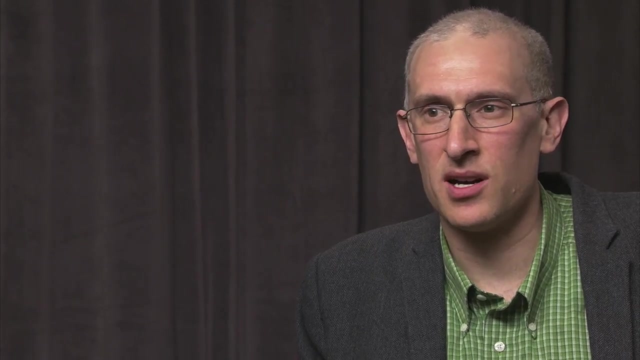 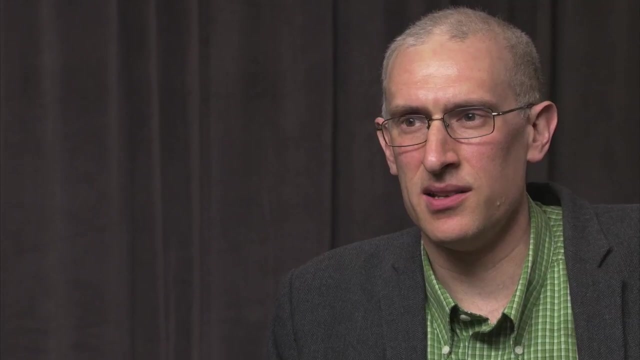 talk to share ideas. ASME, and especially its summer bioengineering conference and now to a growing degree it's nanoengineering for medicine and biology conference, are really fantastic venues to be able to get two or three experts together in your area and have that conversation that. 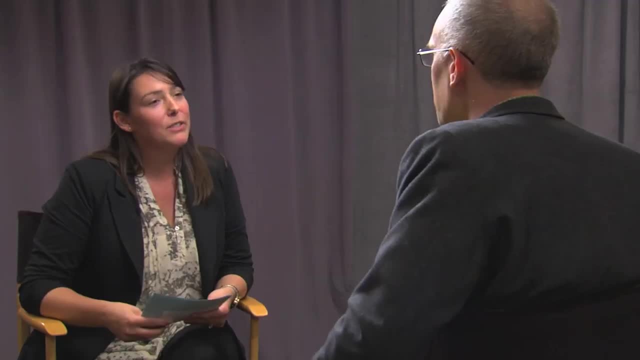 you couldn't really ever have over email or over the phone. Well, Guy, thank you so much for spending your time with us. Thank you for having me here, Alison, Wonderful Thanks.